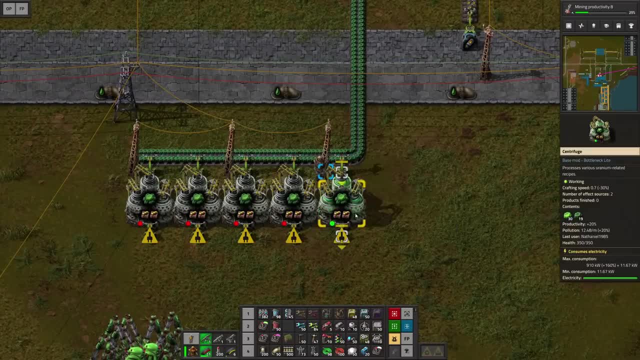 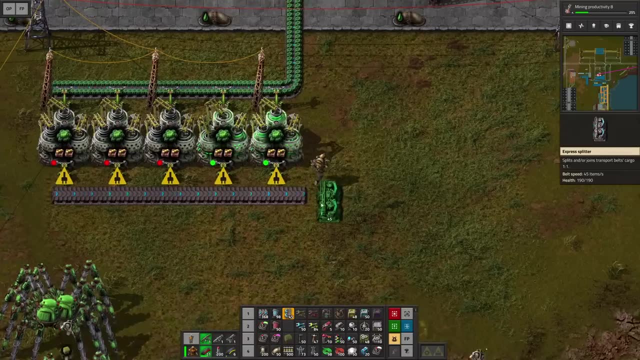 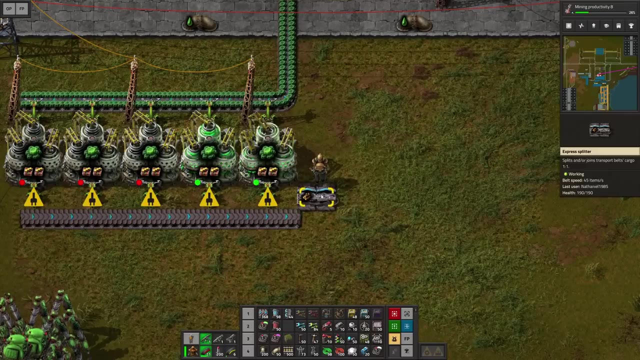 right there. actually, let's grab half of this and give it to the other one. come on, i want two machines to run already. then we're gonna extract them on the other side and let's make sure they actually land on the left side of the belt. so let me see if i just sort out wood on the right side. 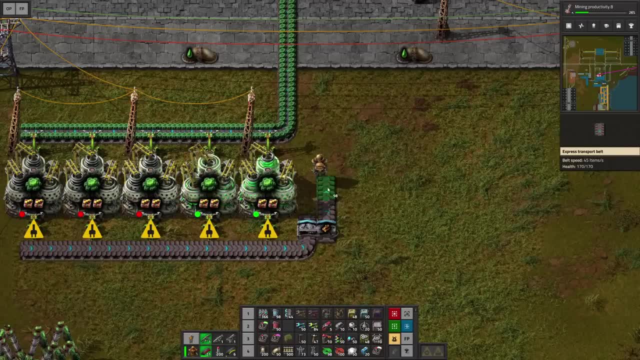 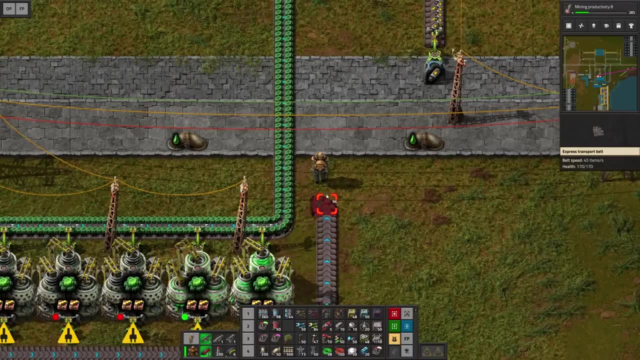 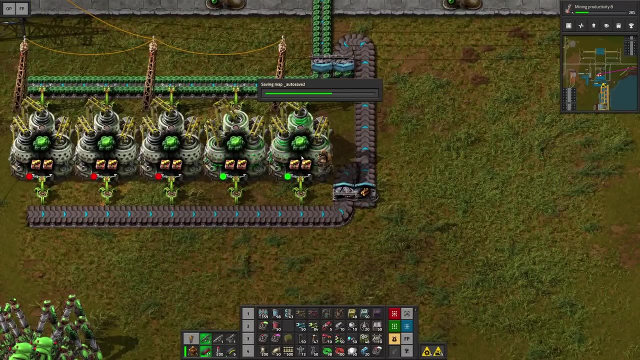 of the belt, then everything else should land on the left side, right, so that means i can make it go to the left side of the belt here. then we're just gonna loop around once, let's go up one more, like so, and we're gonna merge them together. so the stuff that is being expelled here which is 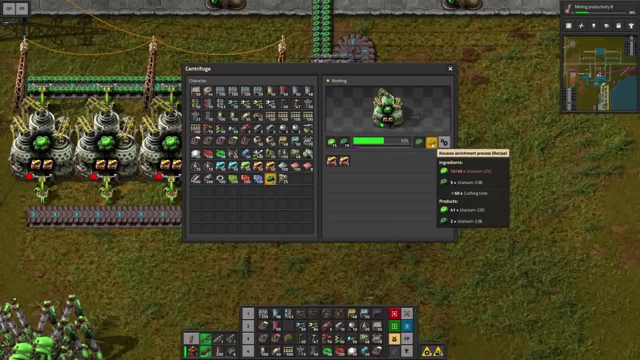 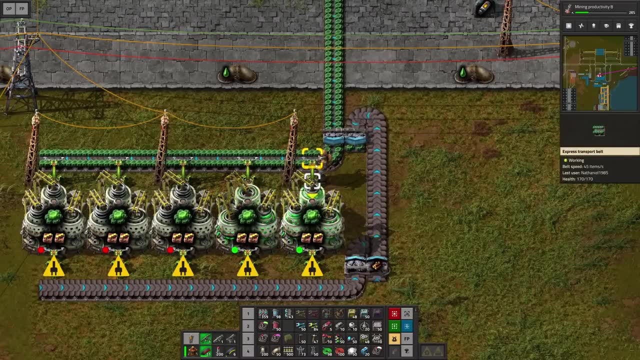 gonna be, yeah, mostly two, three, five, but we also get occasional two, three, eight, and i want them to merge together in here again. the reason i want them on the left side of the belt is because the left side is gonna be the one that is being used up mostly and at the very end we're gonna sort 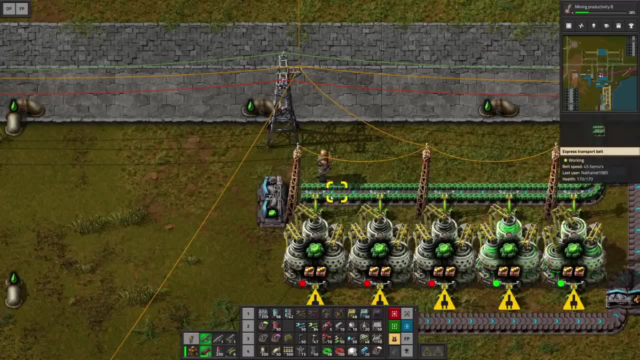 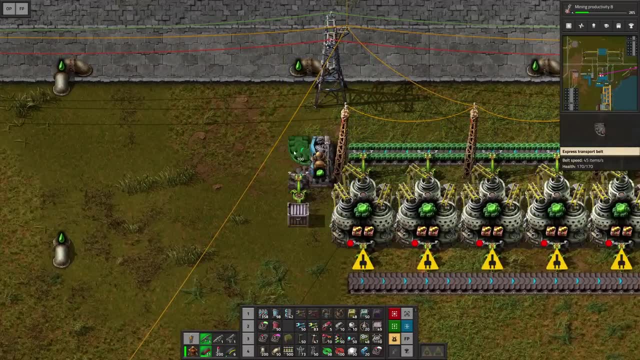 the good stuff out on the left side of the belt and then we're gonna merge them together- side uranium 235- and this will then go down into a storage bin. let's just have that right here and insert it, and all of the other stuff will turn around and then go into a storage system. let me 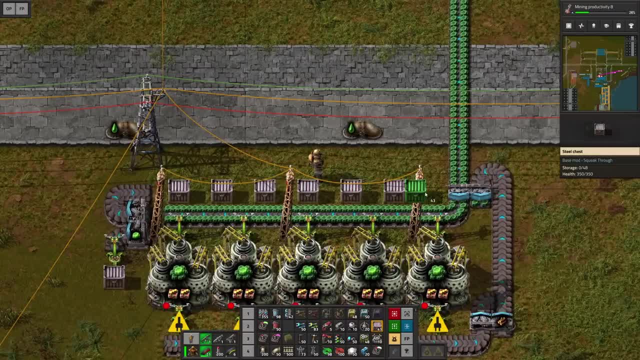 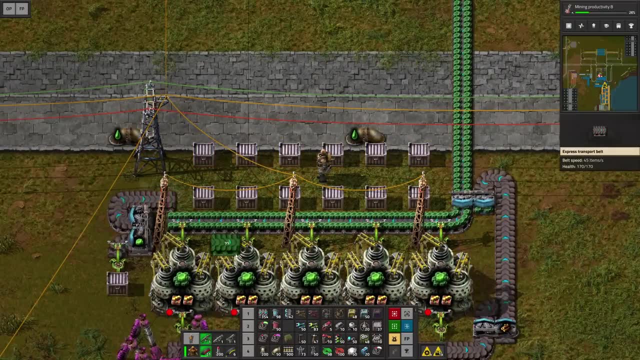 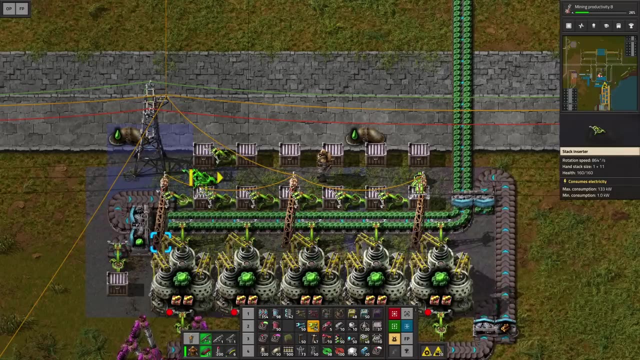 see, yeah, we're just gonna do something like that. i guess let's move that one over, like so. and then i want to add a second row of these. we're gonna go ahead and input them right here, going through all of the chests, and going up, going up here as well. oh, actually, let's remove this and this way. 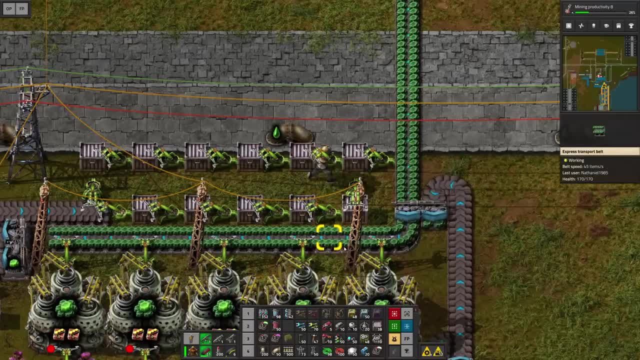 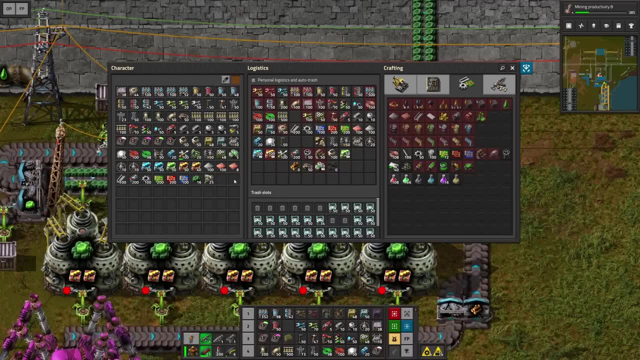 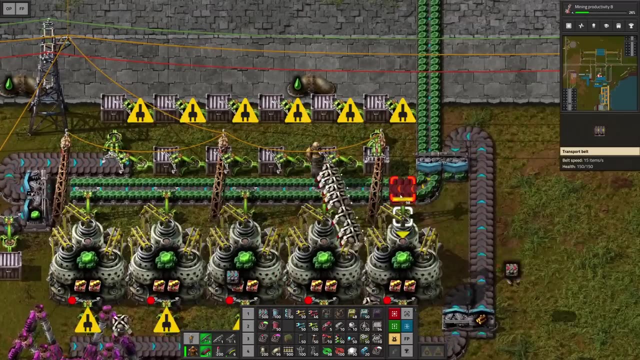 we have two inserters taking care of the picking up part also, i think. to give these guys a little bit more time, i want to swap this to. let's see, oh, i don't have any transport belts. wait, my logistics system wasn't activated. give me transport belts. i want to switch these two slow ones, so the? 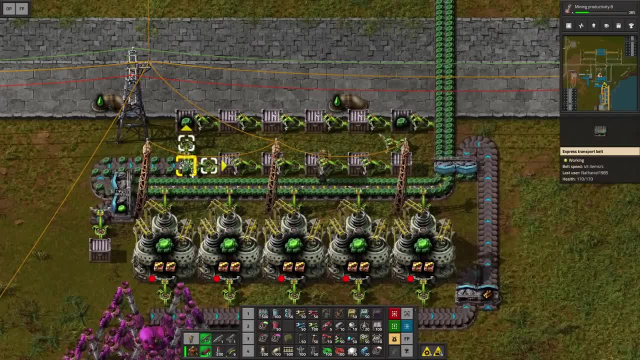 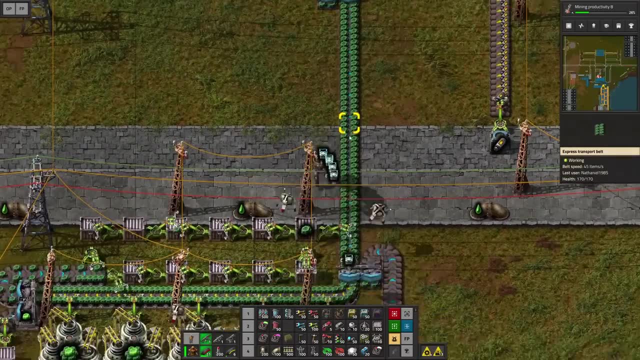 machines have enough time to pick up the stuff, and now all of the bad stuff is being cycled in these chests. I just have to make sure to provide all the power. once we have some space on this belt again, then the items will be recycled and therefore we can use them again and 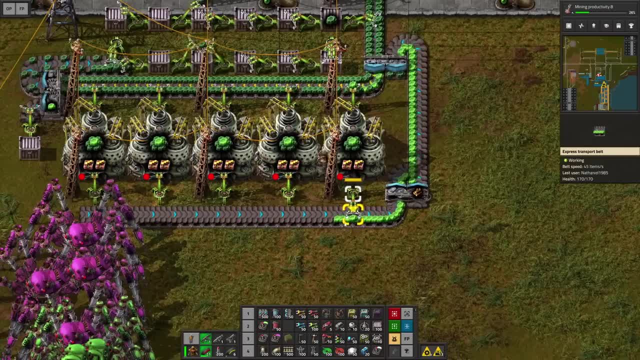 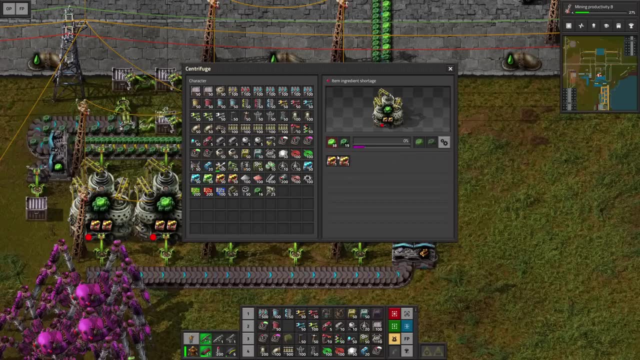 at the moment. yeah, we need power at the bottom whoops, but we can see the 238 being extracted and put back into the machine right away. so that is exactly what I want to see, and I'm gonna feed that again to the next machine. and now some more good stuff is tagging along here. this is good, but 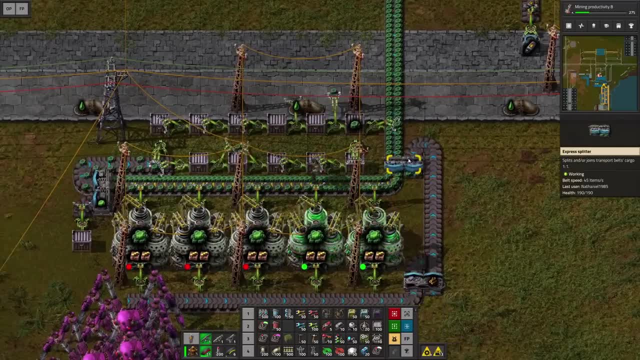 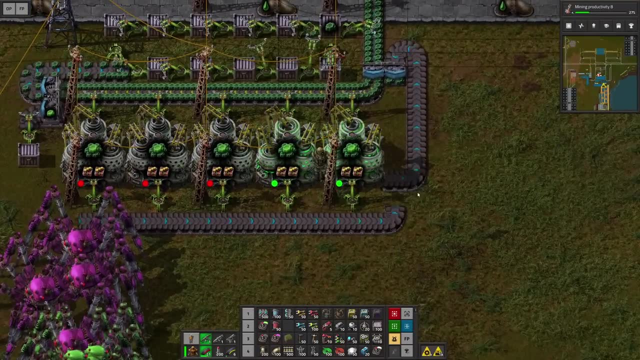 you can see, the left side of the belt is being used up much quicker, though with the two inserters. I have to say we're picking up both rows at the same speed, so it probably doesn't matter. yeah, I think in this case I'm just gonna go ahead and remove that splitter. we can make a third machine. 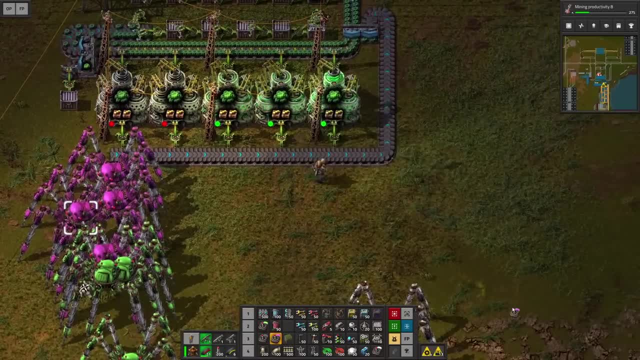 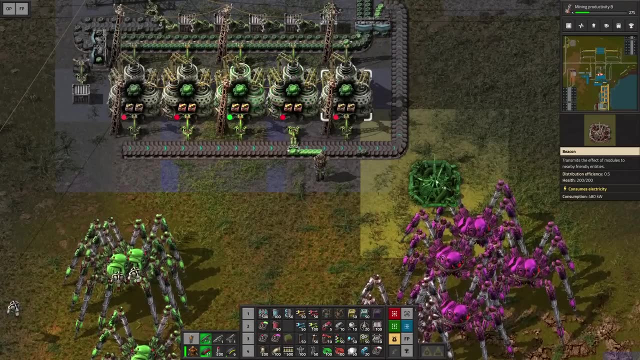 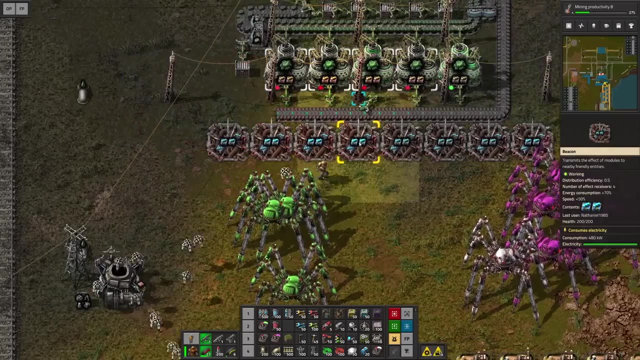 run. that is good. this way we're gonna get the process running in no time. okay, now this is going fairly slowly. my suggestion would be to add beacons. let's do it right here. you get some speed stuff and we're gonna copy the that over. just need some additional power poles, like so nice, that should speed it up quite. 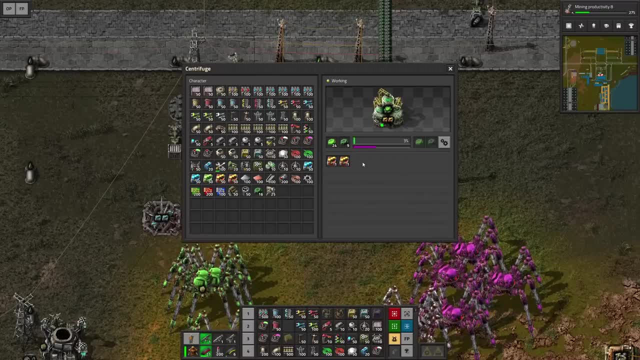 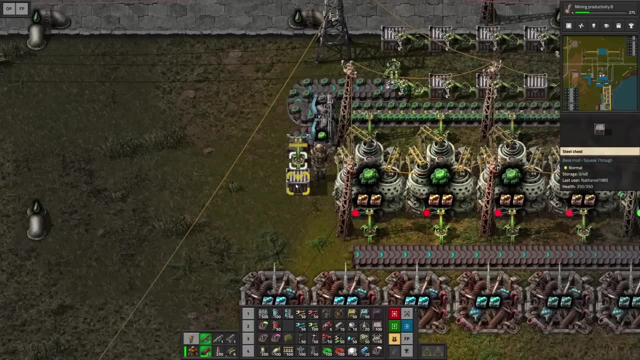 significantly, and we can already take this, distribute it amongst the other machines again, and the idea is that only once all the machines are running at the same time, then we will be getting the extra good stuff that we can then utilize to build nuclear fuel and other things. 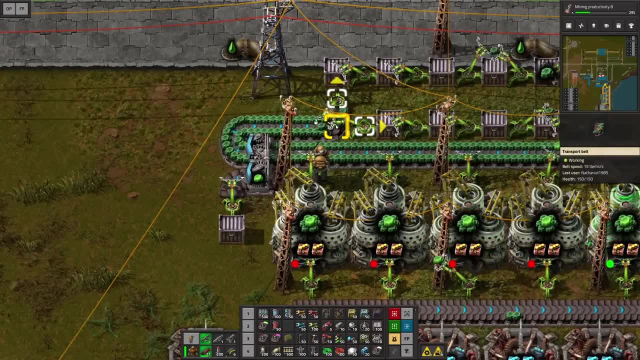 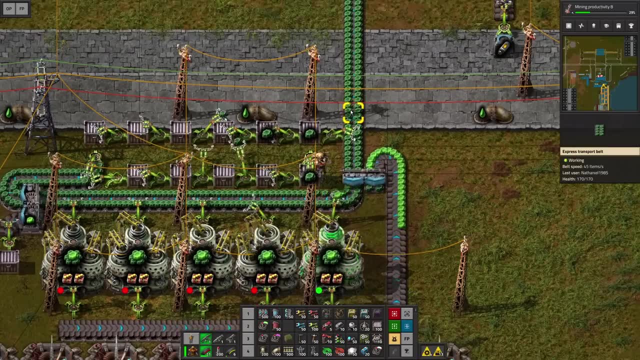 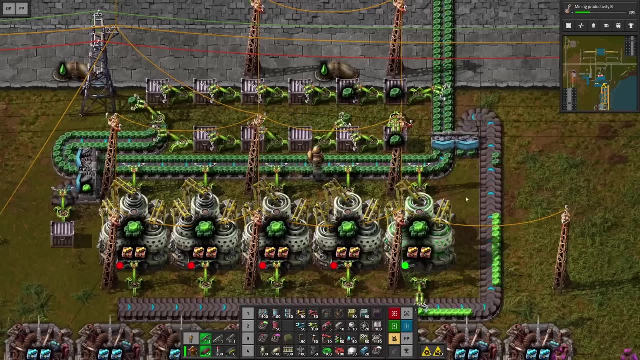 I ended up upgrading the belt again and only downgrading this last belt where the items are being picked up. this has the same effect that both lines are running at the same speed, because we can pick up the entirety of the yellow belt. as soon as I upgrade this say to a red belt, then I think we cannot keep up and you can see mostly the left. 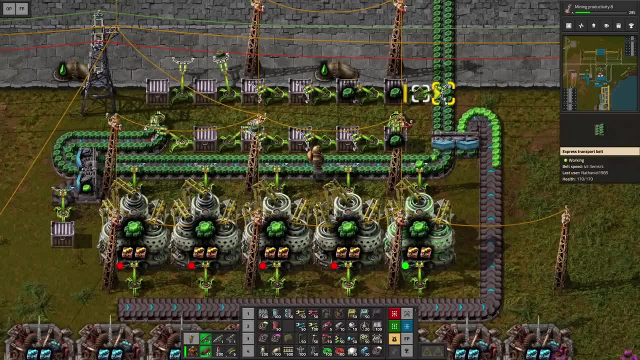 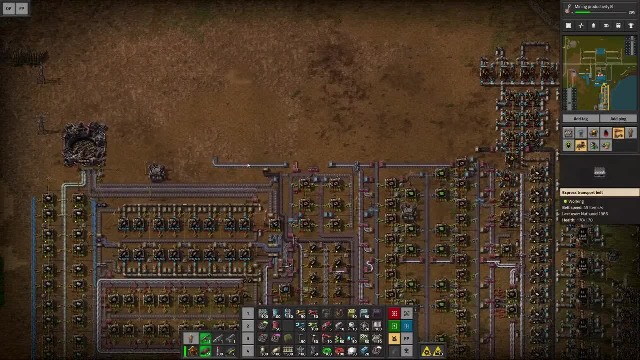 side of the belt running, though it still kind of works, maybe in the beginning. I'm just gonna leave it as such. by the way, I also started taking apart some of the base. for instance, this melting array is already taken apart, and now I'm just waiting for. well, I guess nothing is moving at this point. 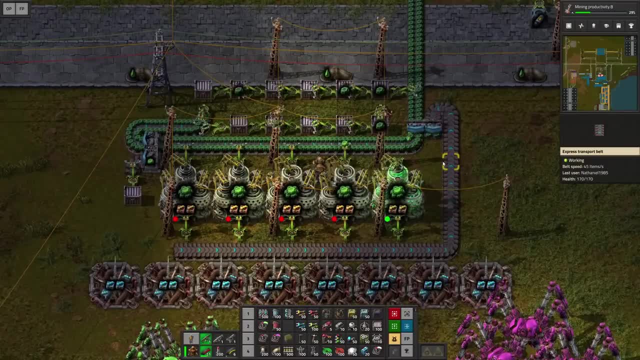 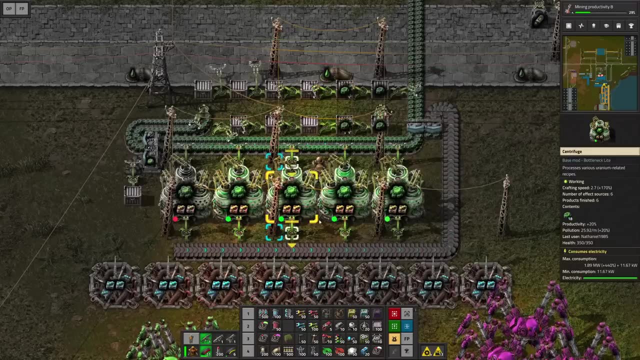 yeah, it's just going really slowly, but I'm just gradually going to take apart the base now we'll see how that goes. in the meantime, I can get my fourth machine running, which is very good. okay, we're back, and it took about half an hour. I sped it up by actually. 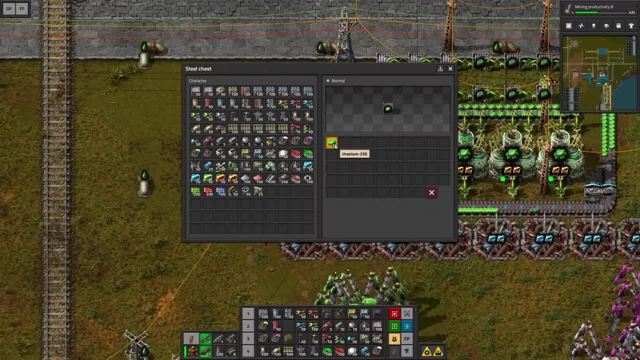 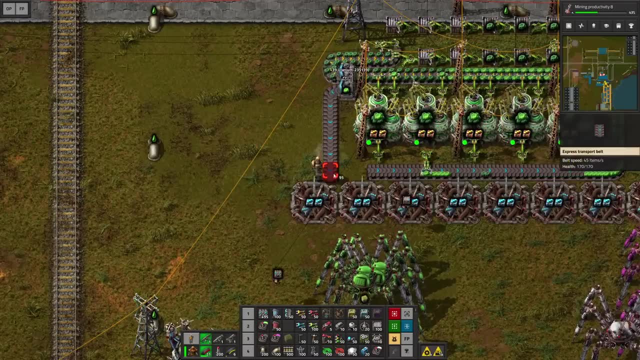 babysitting it a little bit, but now we got our first output of uranium 235 that we can use for whatever we like. so my suggestion would be to actually continue this along here and then we can set up another production line, maybe do something like that. okay, the nuclear fuel. 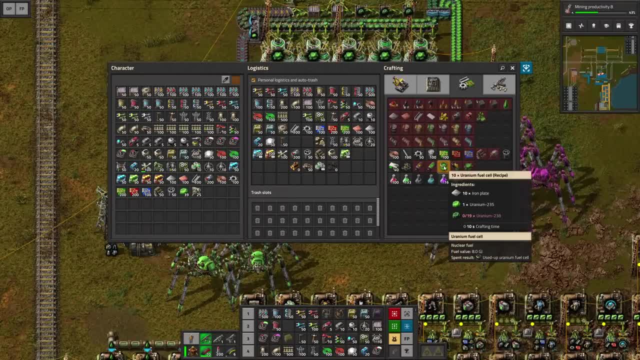 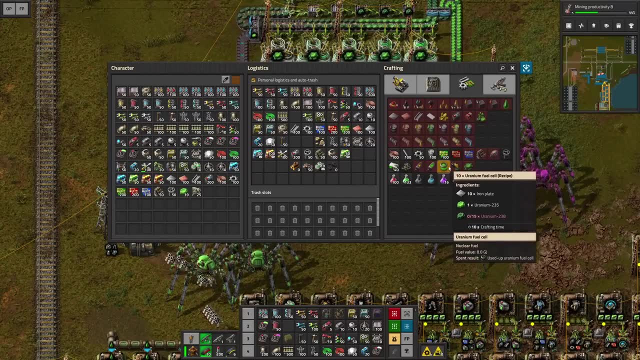 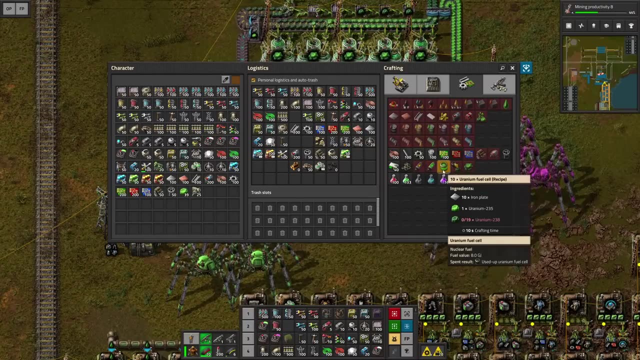 is made in the centrifuge just using one uranium, and then the uranium fuel cell will also be using 19 uranium 238. the uranium fuel cell at the moment is more important to me because the power issue is more pressing. at the moment we're using rocket fuel for the trains and that is just fine. so as 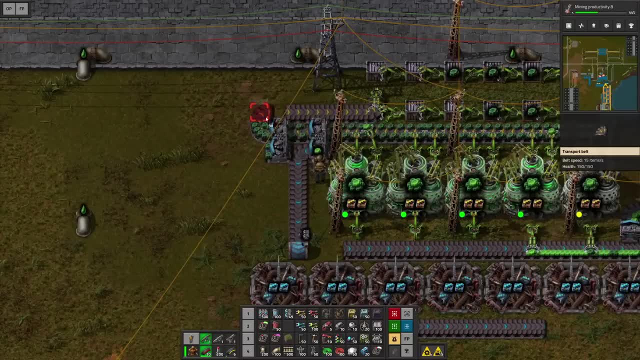 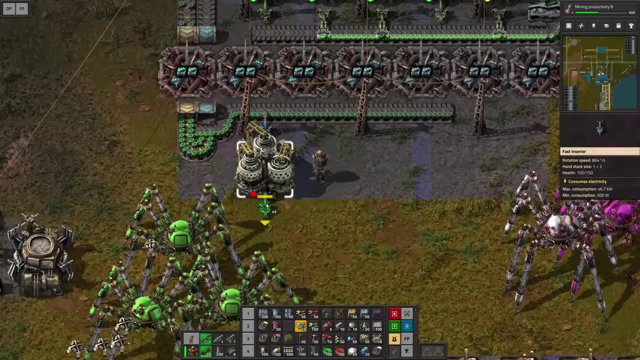 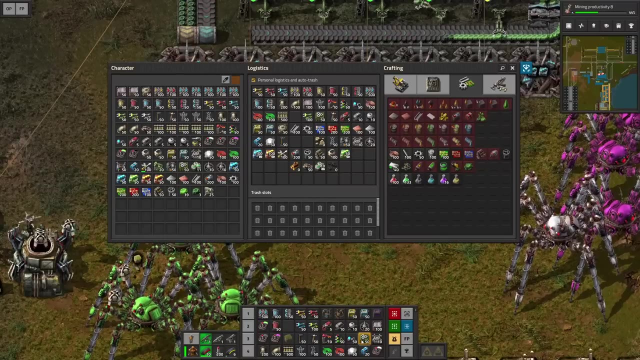 a matter of fact, we need to expand this slightly, do something like that in order to gain access, and I guess we can go ahead and combine it as such. yeah, then we just need to add a bunch of computers here and we should be getting the nuclear fuel. no wait, that's wrong. the nuclear 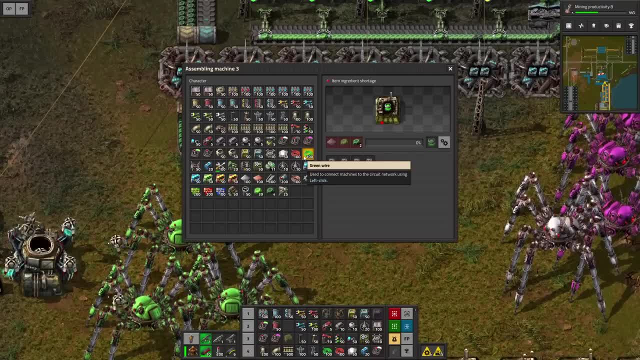 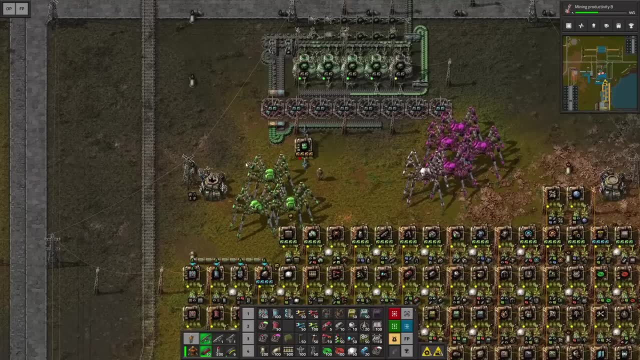 fuel is made in an assembling machine. okay, so uranium fuel cell. that's what I want to craft here. can I do productivity wonderful? oh no, we also need iron plates. what a shame. but we are inside the logistics Network so it's not a problem. but that means I want to request a couple of iron. 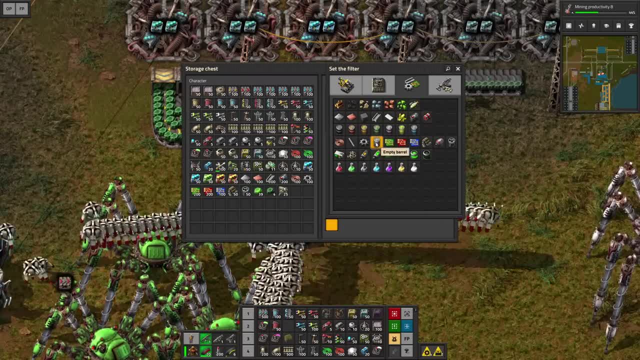 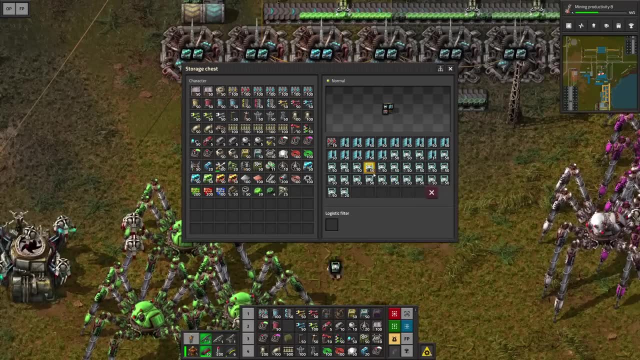 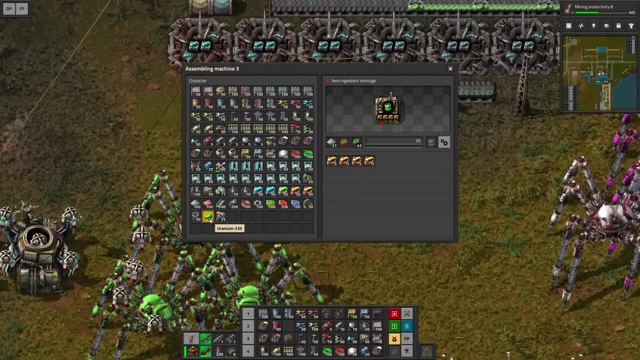 plates as well, and then why not just go ahead and output that here into a storage bin? oh, did I just? yeah, I just made a mistake there. I still had a bunch of accumulators and stuff queued up there. no problem, I'm gonna take that back and maybe put it into my spider-tron. for now, I'm gonna input the. 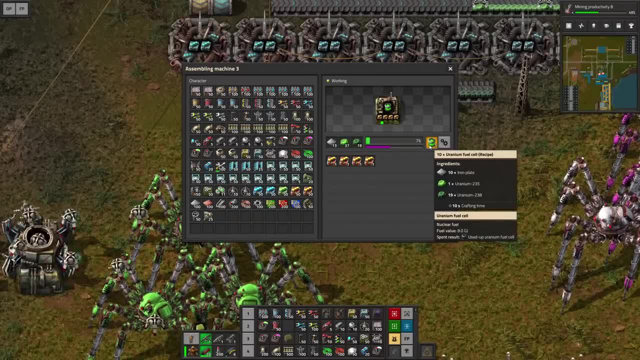 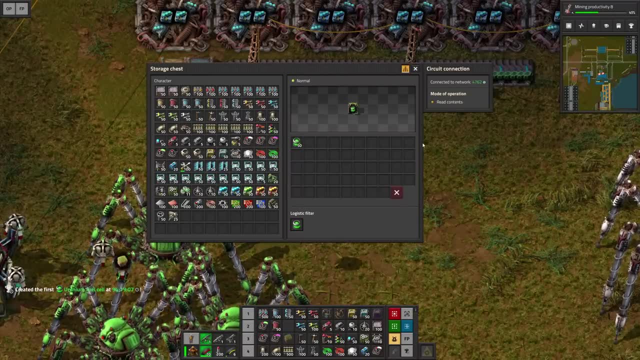 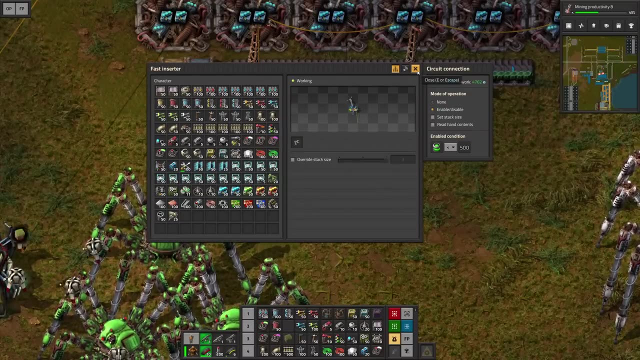 uranium myself for the time being, and now we are creating the fuel already. nice, I'm gonna hook that up to some cabling. let's say we want to store at least 500 of these, so I'm gonna set that in the filter. I could also set anything. now it's gonna craft 500 and then it's gonna stop. 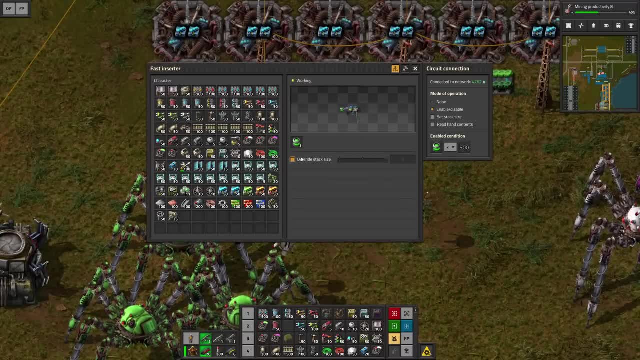 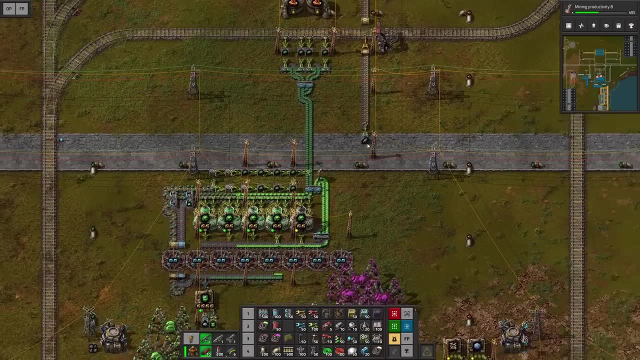 wow, this is creating a lot of fuel cells in a short amount of time with just a few materials. this is actually quite insane. I don't think we're gonna need more than one machine, honestly. okay. now the question is: how are we gonna ship this over? let's say we have our nuclear reactor somewhere. 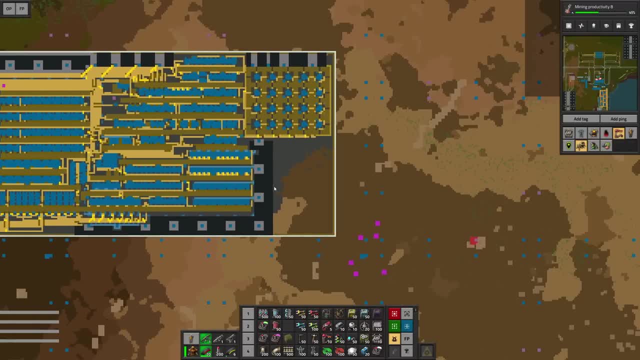 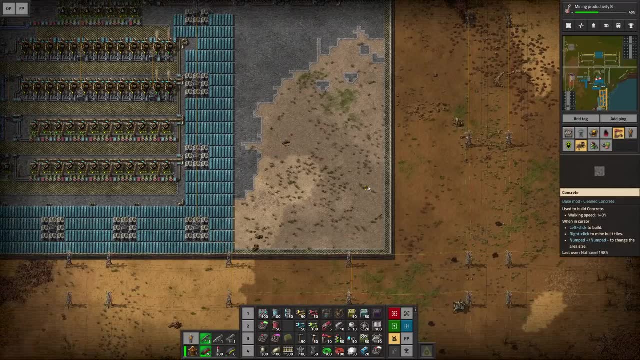 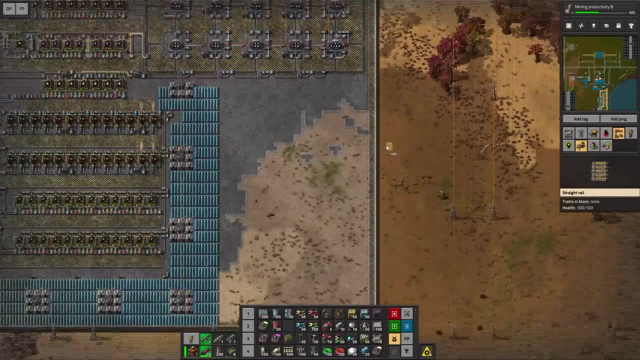 here I might actually have to make a little bit more space to accommodate for everything. but that means we have to bring the fuel cells here and we also have to get the empty fuel cells, the used up, back. we could theoretically just move this over, move the train along here and then have a little 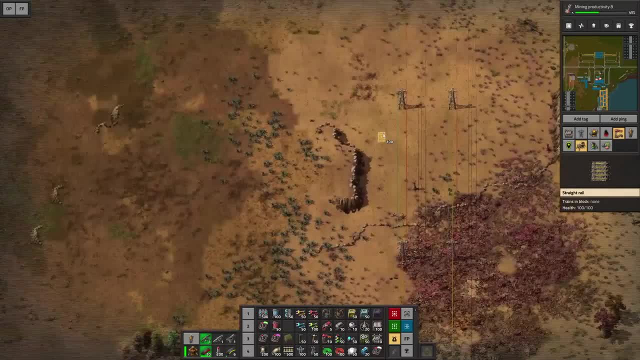 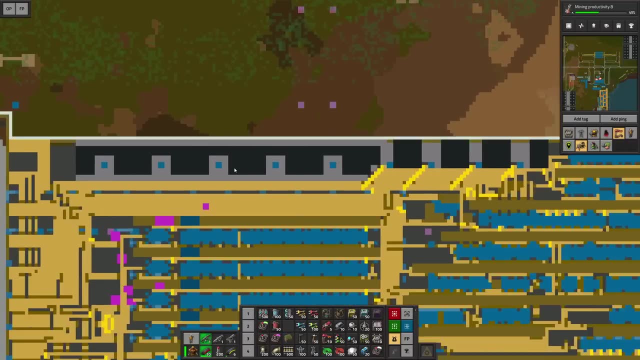 station to drop the fuel and we can then go ahead, join back with the train tracks right there. I like this idea. so we would be moving the wall up a little bit and then just fill up the gaps with solar panels, but you know what that means. we can also go ahead and make nuclear fuel already. I 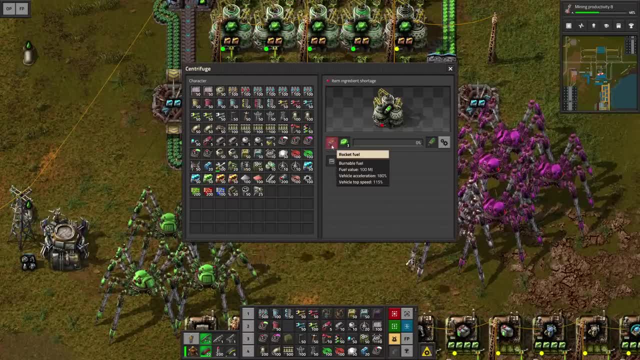 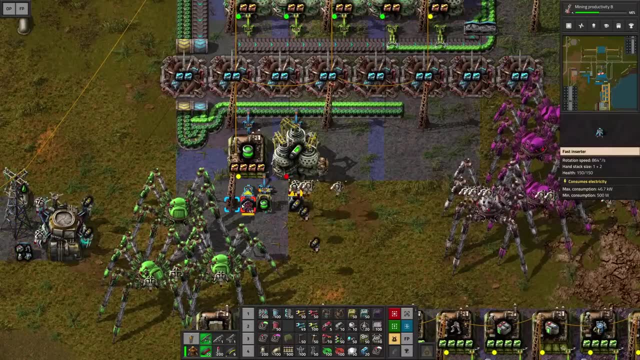 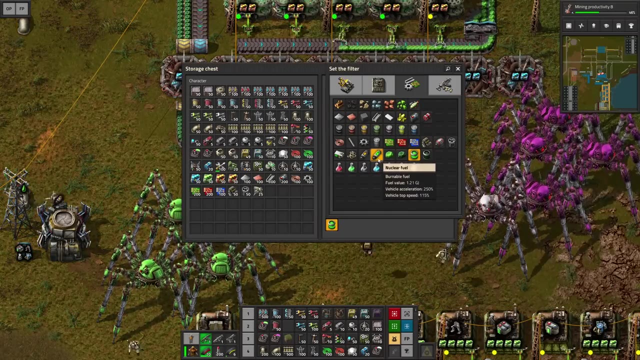 mean, if we are over producing the 238 already, we need some rocket fuel for that. we can get a requester chest asking for that. let's get 100 pieces and insert these guys as well. okay, very nice, let's get a storage chest, nuclear fuel also. want to hook that up to a cable and we are gonna set this to what? 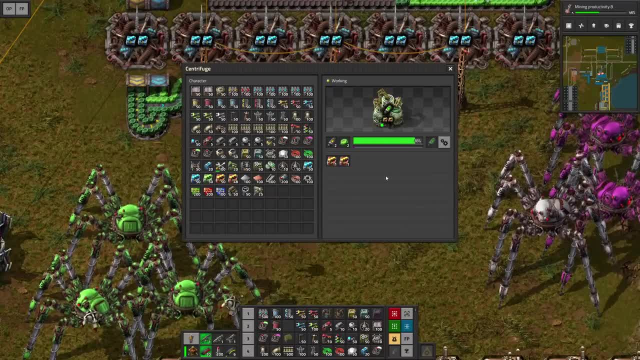 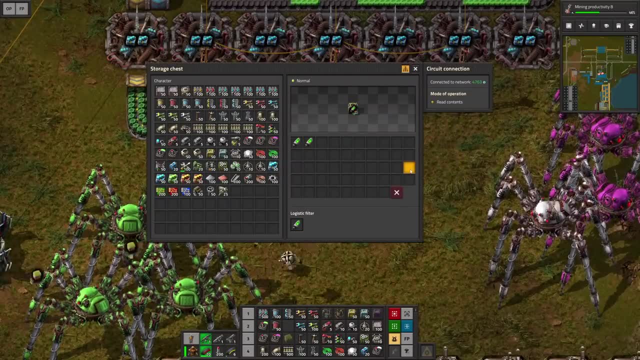 now the question is: how much is this gonna stack? yes, of course we want to use productivity honestly. it doesn't look like it's gonna stack, so that would be 10, 20, 30, 40.. we cannot get 50 in there. let's do 40.. good, that means. 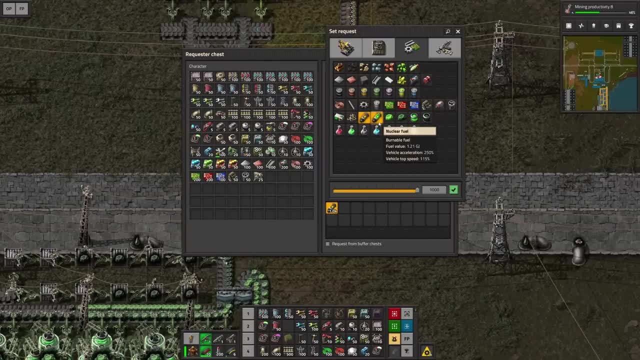 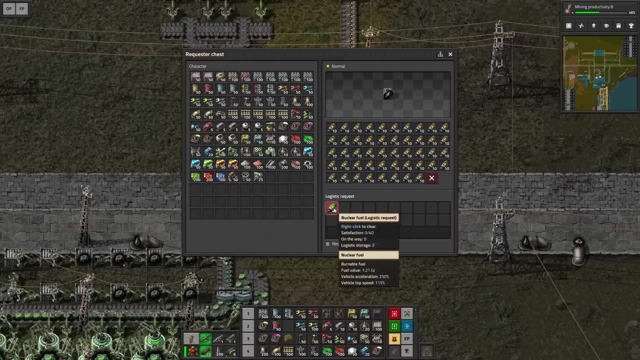 we can already go ahead and change this here. yeah, this should now be requesting nuclear fuel, and we want to do 40 as well. I will still be using up the rocket fuel here first, but afterwards we are gonna switch to nuclear fuel. this is pretty dope, I have to say. I think I'm gonna set up one more. 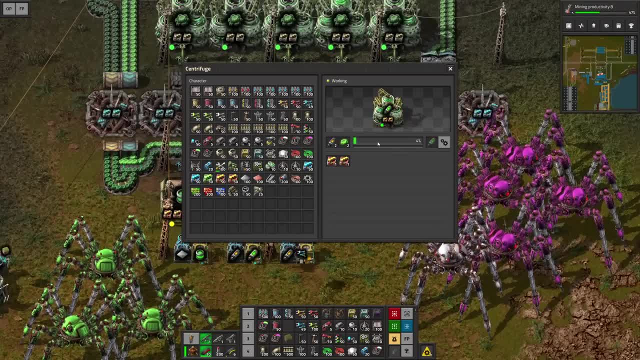 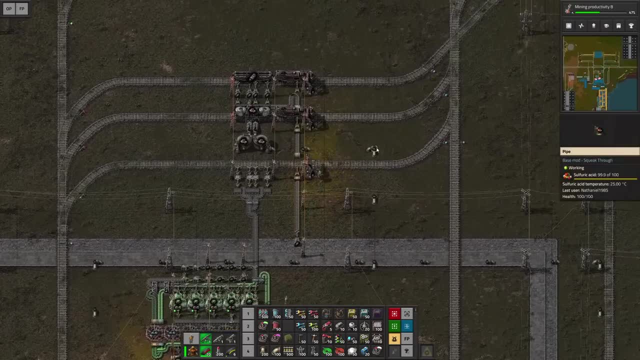 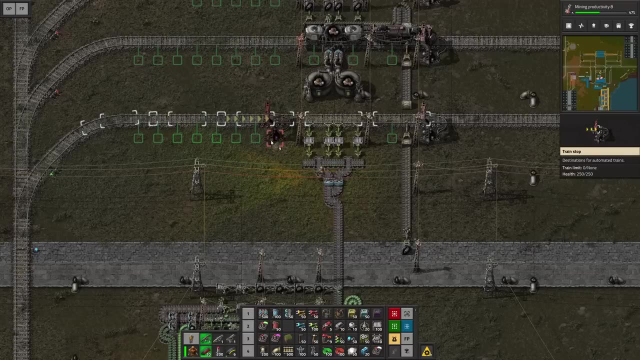 machine for this, get an inserter here, and this way we are crofting double the amount. the uranium fuel cells are already crafted. that means we now need to take care of the fuel station. we could do it a train for a very long time in this region and that means i could set up another station enable 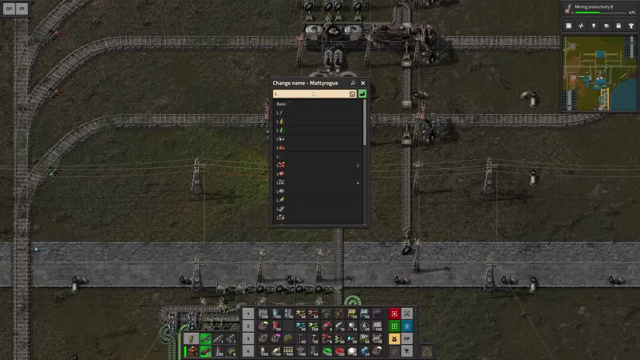 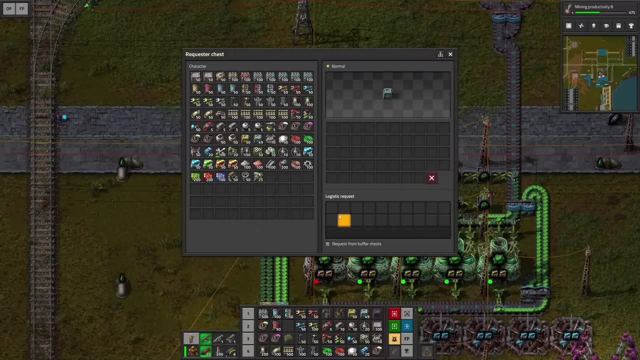 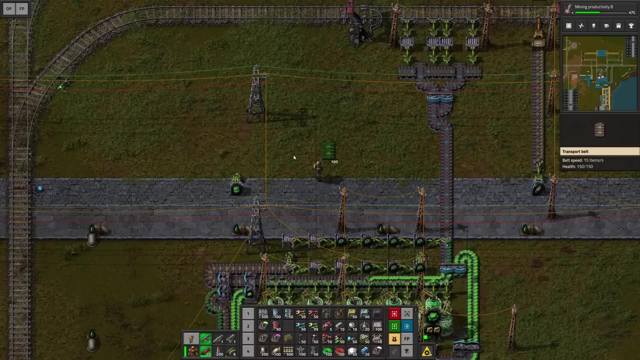 train limit of one and i would be naming that load. where is the fuel cell? right there. that means we can take our requested chest, for instance, right there and request those fuel cells. let's do two stacks, uh, come on like so and we're gonna exporting them over here and introducing them into the train. 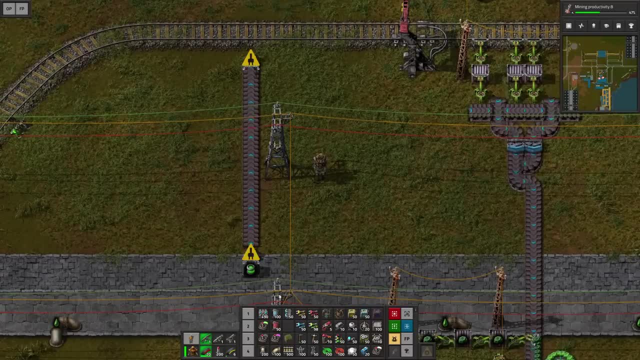 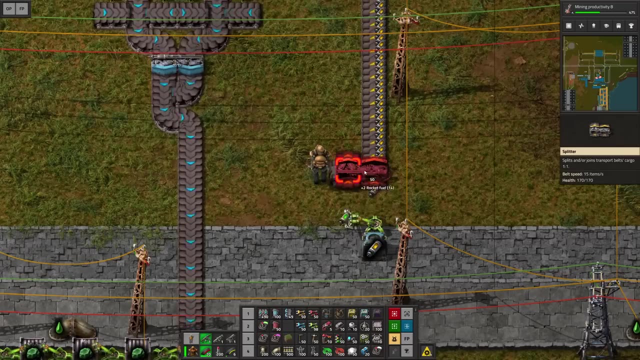 actually, let's use a blue belt for this and also: uh, this is gonna land on the right side, we're gonna fill up the entire belt. let's also do that right here. oh, actually that's not gonna work. we have to place it one later. we already have some nuclear fuel here. that is good and bad at the. 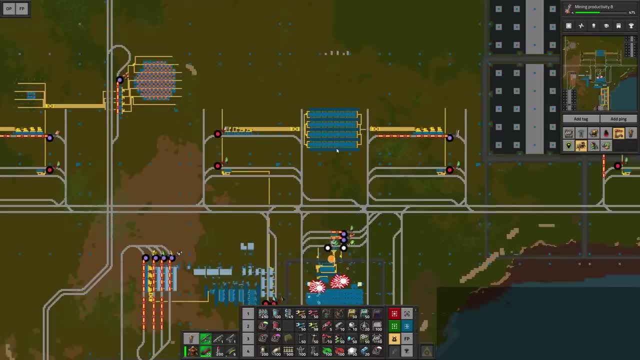 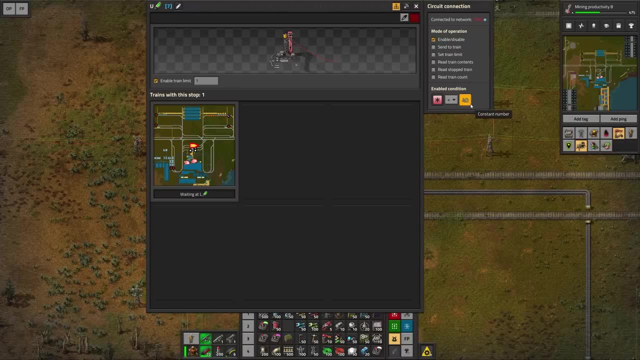 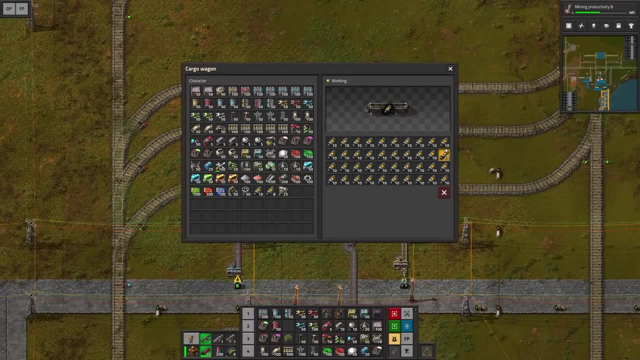 same time, because we cannot request as many. hmm, let me think at the moment we are requesting 100, which is way too many. let's go down to 40. okay, that's just crazy. i mean i don't want 40.. wait, let me think how many will be delivered at the time. we have the space for 40.. so that means 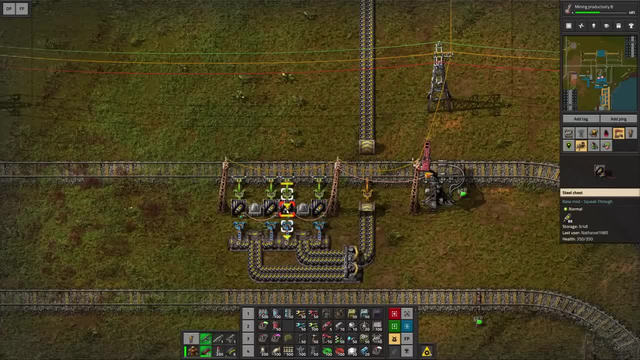 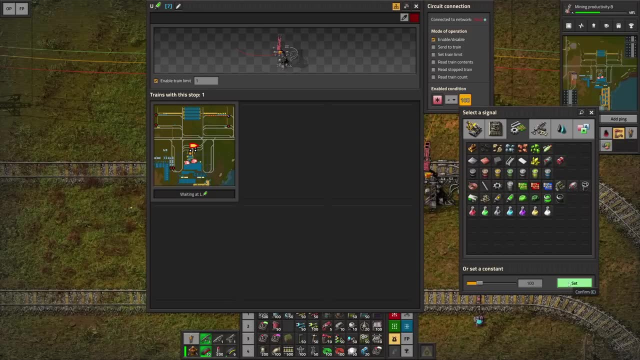 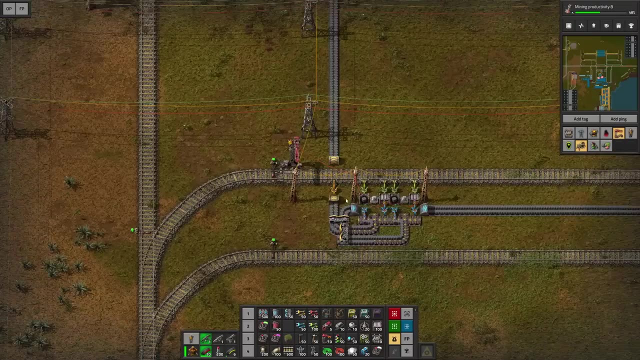 40 are being delivered. we have four chests, each of them having more space than 40.. okay, that is actually good. that means we're gonna request a train when we are at 100 and we can keep it at the setting we have it currently at. okay, i like that. it's gonna be a lot of fuel that we ship over. 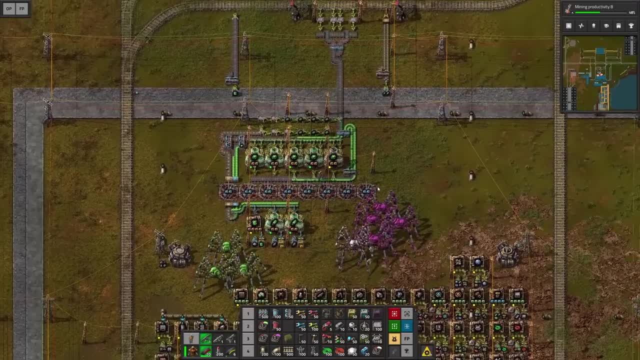 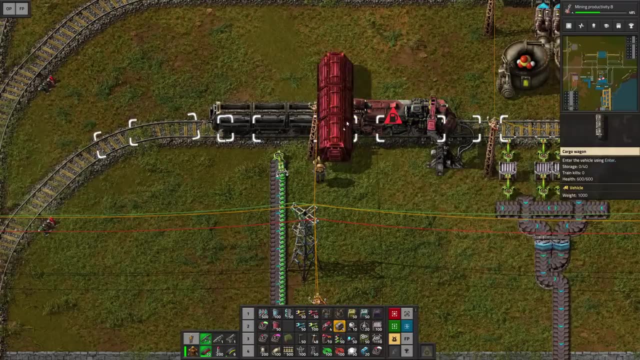 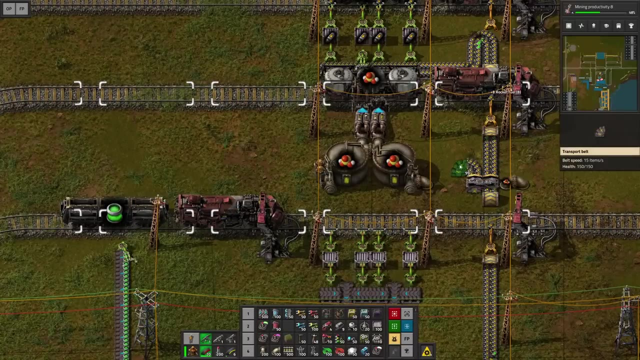 but i think we're gonna be fine, considering we're already crafting a bunch of fuel. well, i guess of it is landing in here. that is fine. by the way, we need another train here gonna set this up and, oh, this also needs to be fueled. um, i think i'm gonna do it from this side. 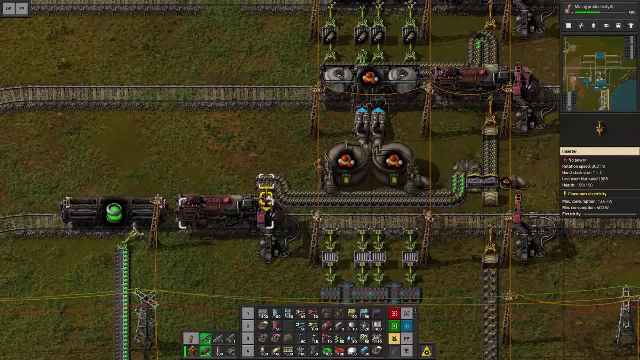 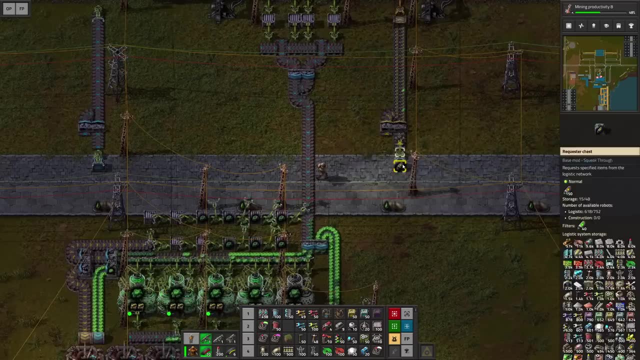 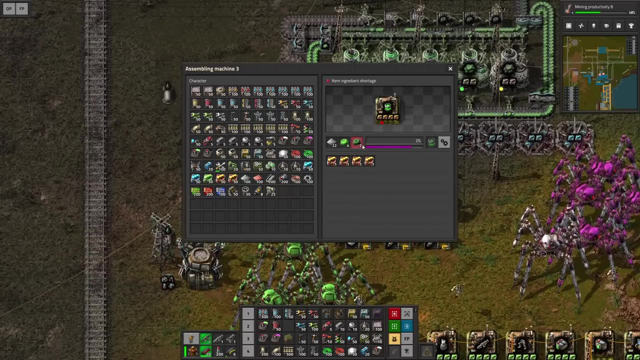 this seems to be the easiest, and now i can fuel this guy up as well. i know i thought i had this one covered there. let's fuel it up over here then. okay, it's so funny. now we just have the occasional nuclear fuel already going into the system. wait a second. what are you doing? why are 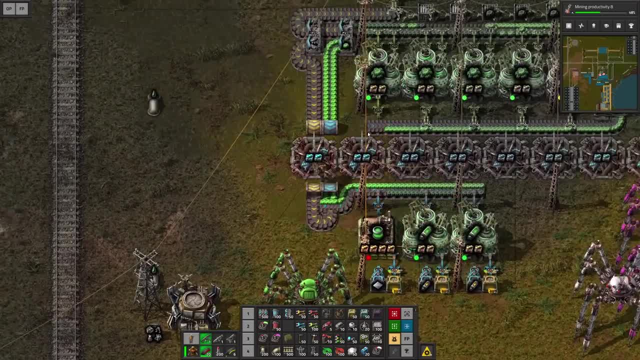 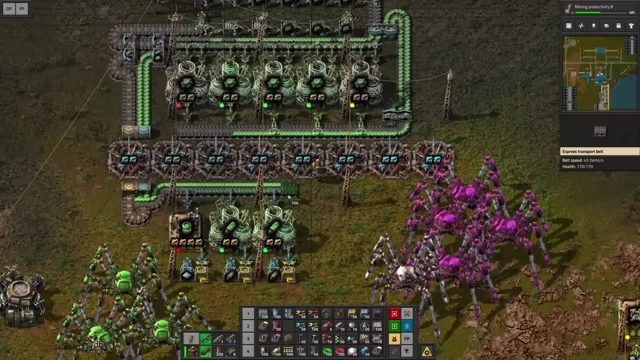 you not? oh no, i mean, you should do this. uh-oh, what is this? um, uh-oh, okay, uh-oh, okay, what is this? of course, what is this? um, uh-oh, okay, okay, okay, okay, uh-oh, okay. what is this? uh-oh? 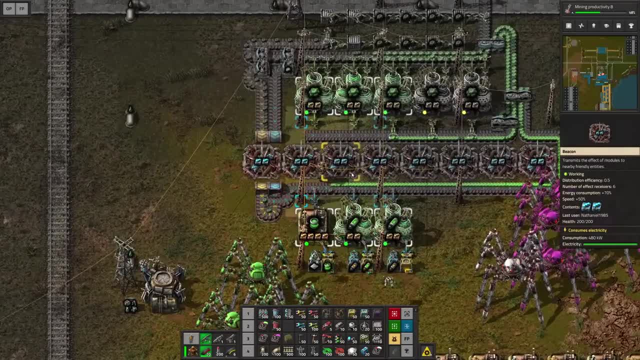 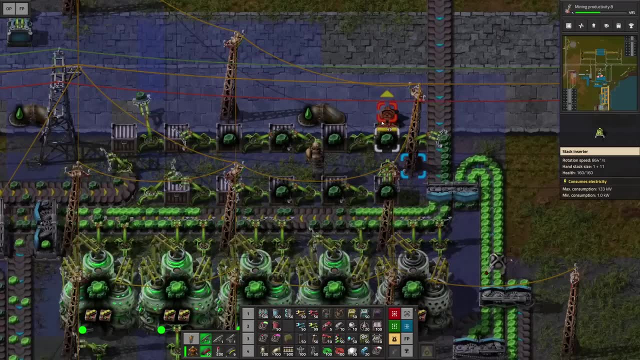 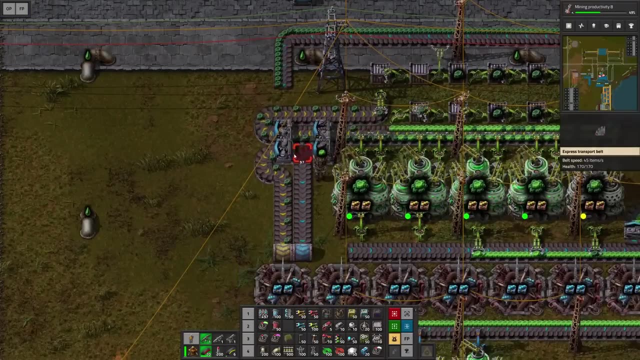 okay, i was, i was oh, okay, okay, so you know, this is it. it looks like it's not really like like a, like a. there looks like like a um, um. okay, it's okay, so elegant, but just to test things out, I'm gonna change it if it works out. but instead of doing 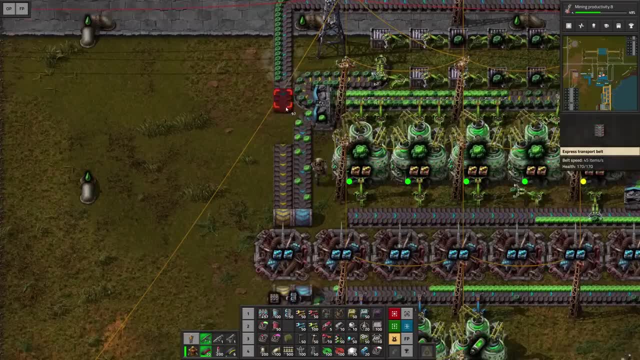 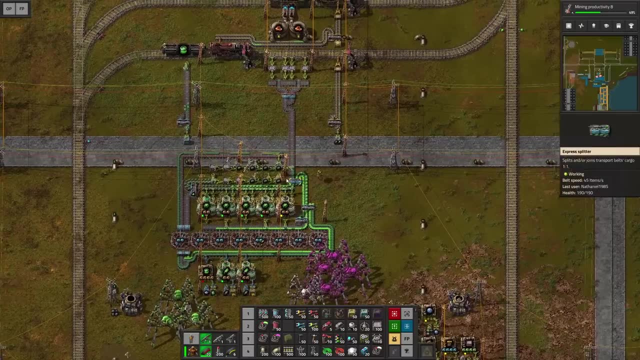 that. so we're just gonna remove this connection, we're gonna utilize this connection and therefore we now have a really good supply of 235 as well. yeah, I think this might actually work out. let's leave it be for a little while and check this out. okay, where does this need to go? now it needs to go. 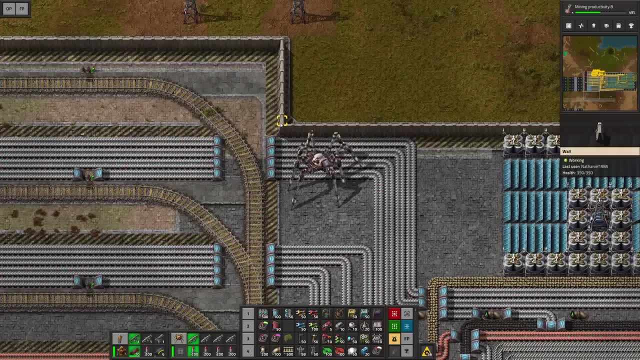 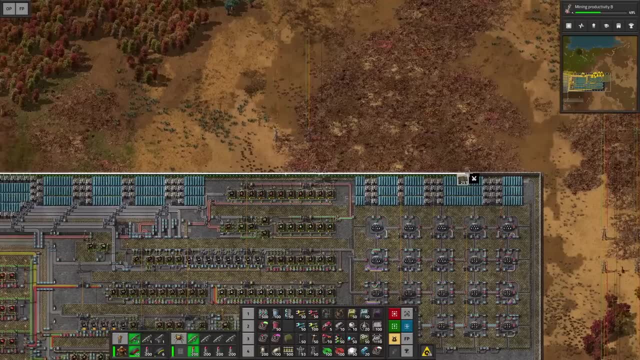 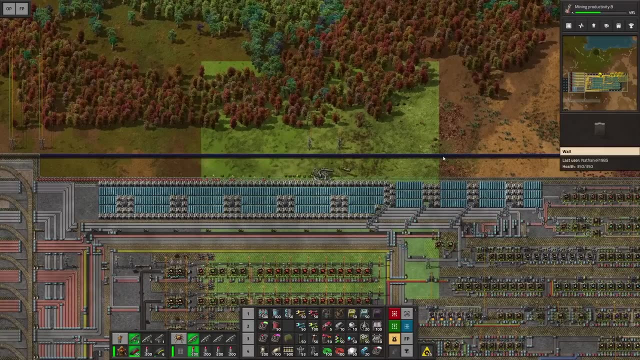 over here. let's call our spider and make our way over there. in order to accomplish this, I wanted to move the wall. actually, maybe we can just cut this out. yeah, get this entire wall out of the way. whoa, that's a big, big wall and I'm gonna attach it right there. then we could take this rail by. 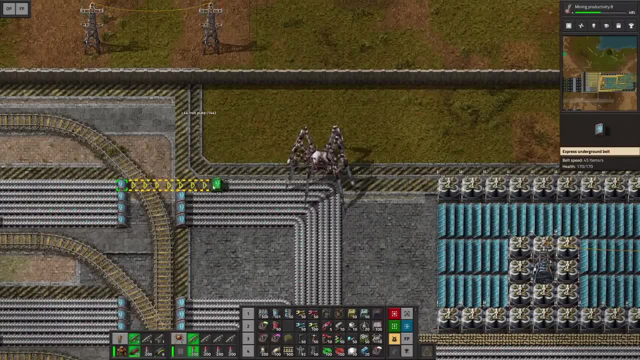 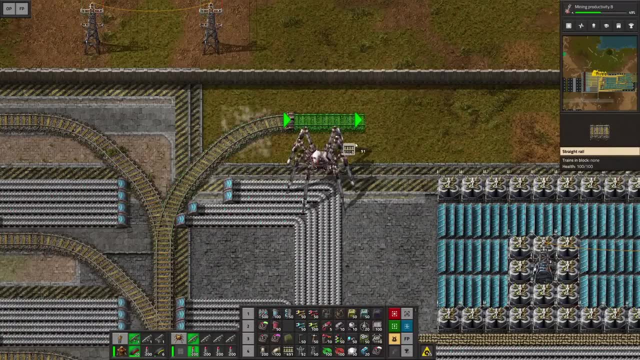 moving these guys just a little bit, or as far as they can go. I think this one too, and that might already be enough, right? no, this guy is in the way. now we can do it. okay, let's move them just as far back as they need to. yeah, like that. 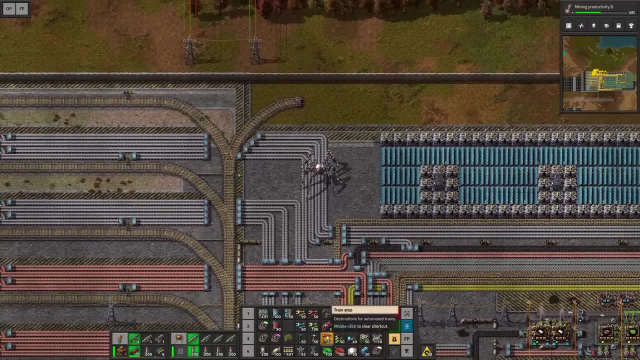 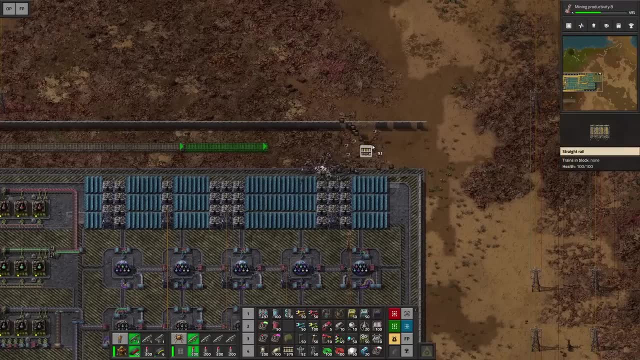 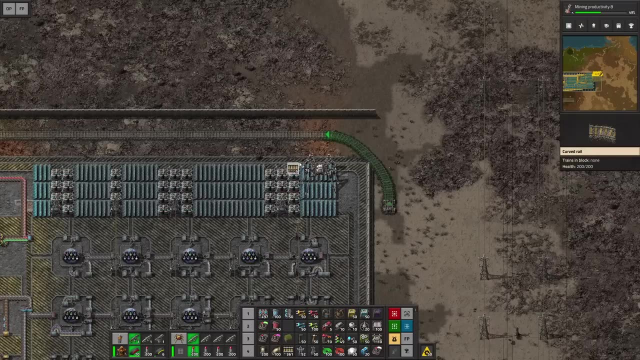 this is good. I would then add a light here and a rail signal there. actually, this light is not necessary right now. let's go ahead and continue the rail, and we're gonna make it all the way over here and try to cut into the lower piece there. I want to end up approximately here. yeah, that should. 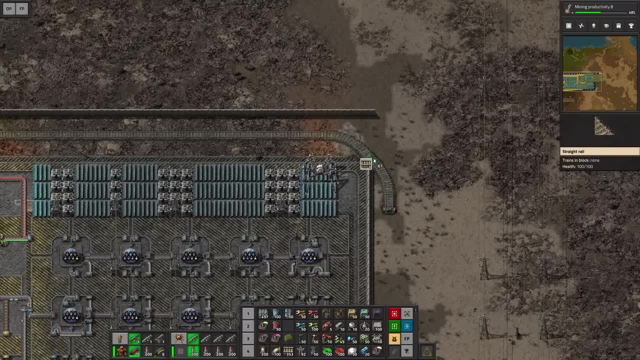 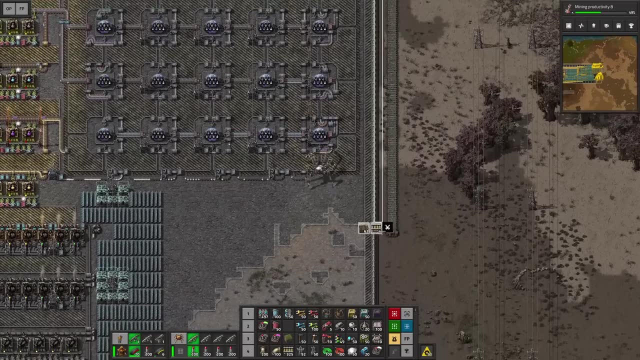 be good, right? oh, this is not connecting, wait, like so? okay, then it can go down and somewhere here we have the station kind of also makes me want to move this wall, and we might therefore also have to adjust the flooring. actually, the flooring is still good since the 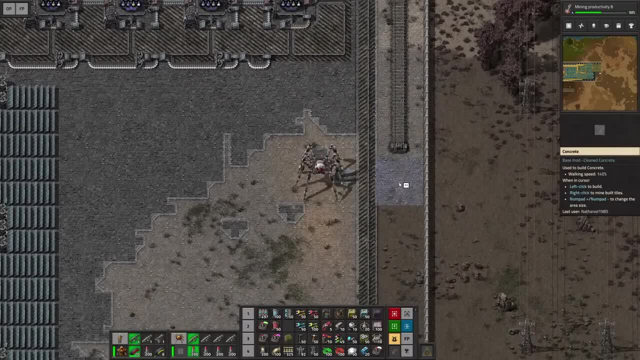 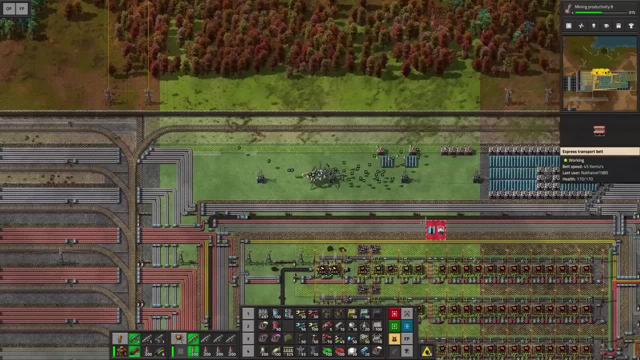 track is kind of going along here. however, I want to see some concrete beneath the tracks here as well. okay, this is looking good so far, but for now I'm gonna remove the solar panels and accumulators. I will be finding a more suitable pattern now with the track and everything. as a matter of fact, I'm 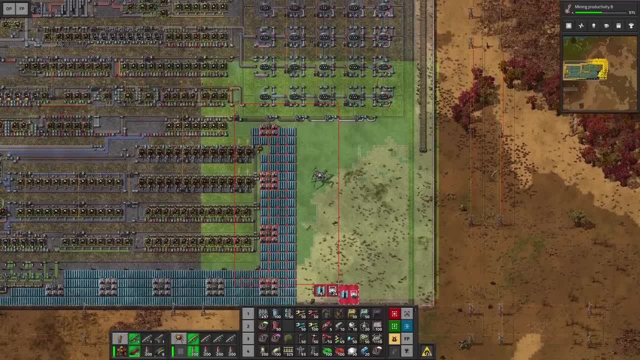 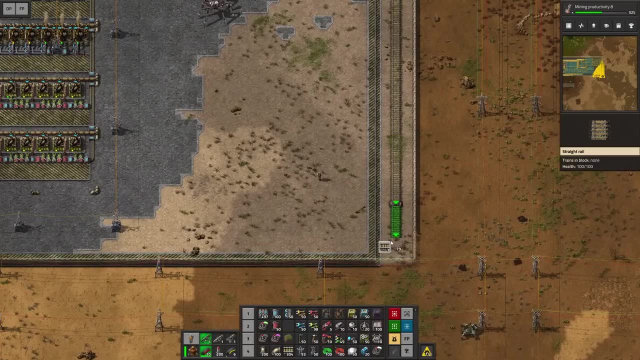 gonna do that for the entire module where I have placed them. so here all of these can go as well. yeah, yeah, yeah, I'm gonna redo that once everything is in place. the idea is I'm gonna deliver the fuel cells and get the empty fuel cells with the same. 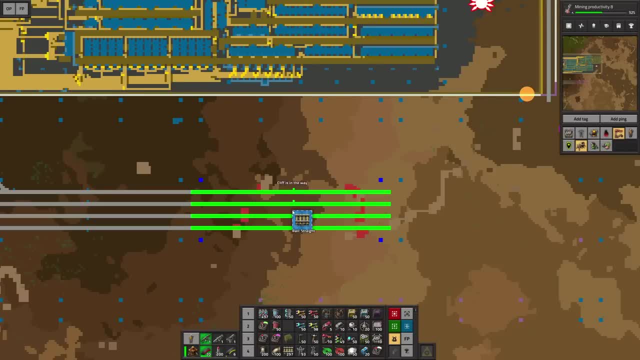 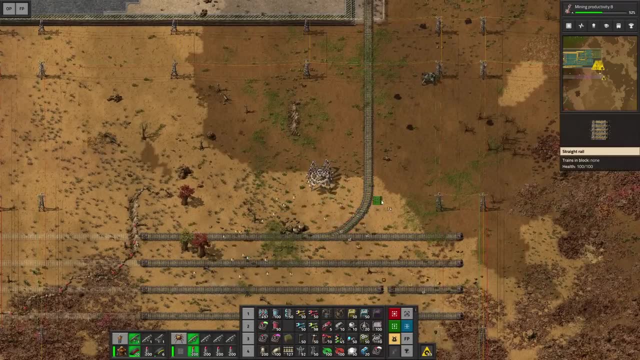 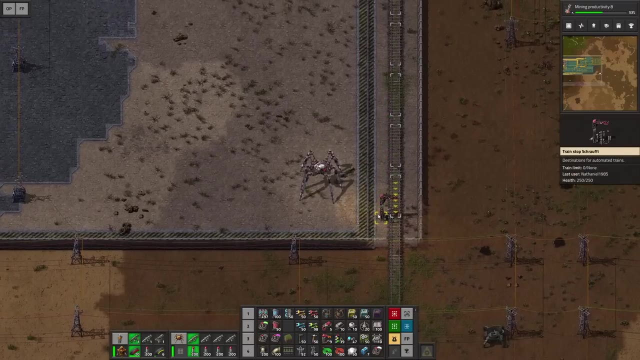 wagon, then we're just gonna escape right here and we will be going down back into the tracks somehow. so, going down here and then either joining up with this rail or joining up with the next one, now let's see if we can set up a station here. I mean, well, we can, should be fairly. 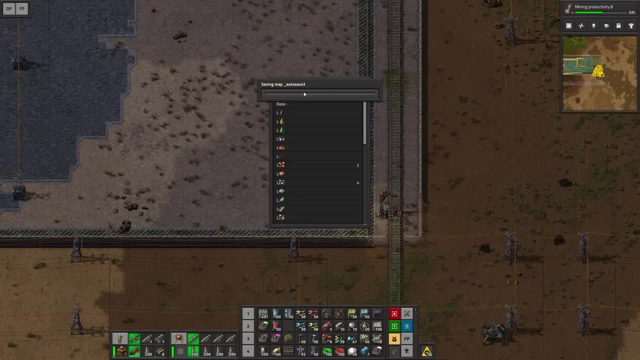 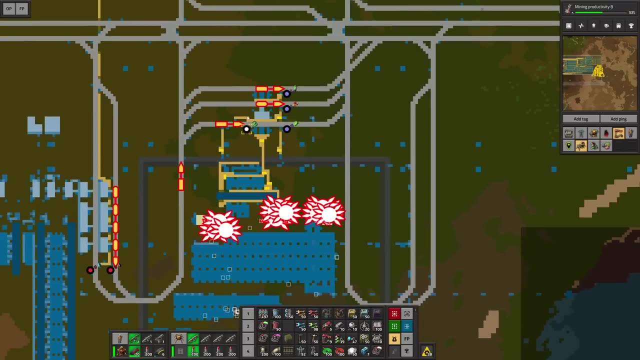 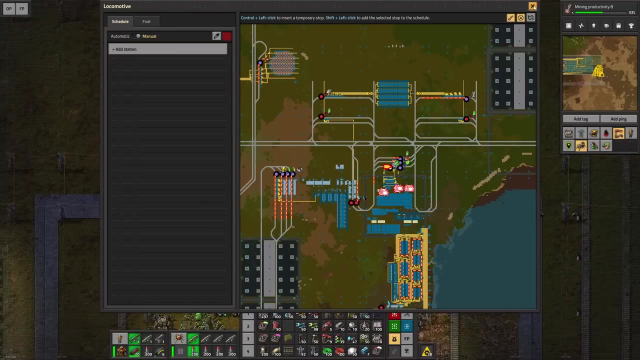 obvious. but you know, enable train limit of one, and then this is gonna be unload a fuel cell right there and we apply this change. okay, if we then have a look at the train we created previously, oh, this guy now has to wait. yeah, I'm, we get this guy running. that is actually a potential problem. 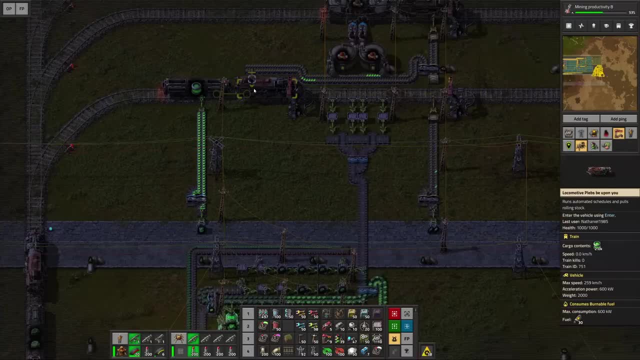 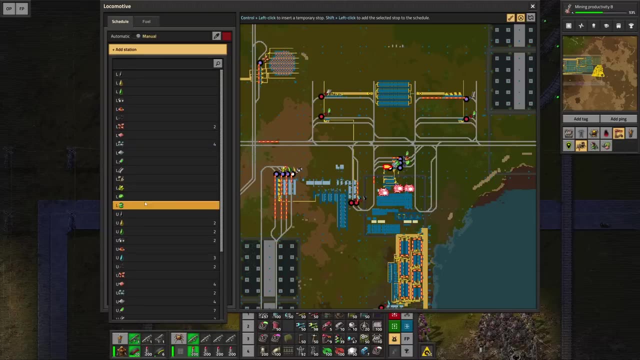 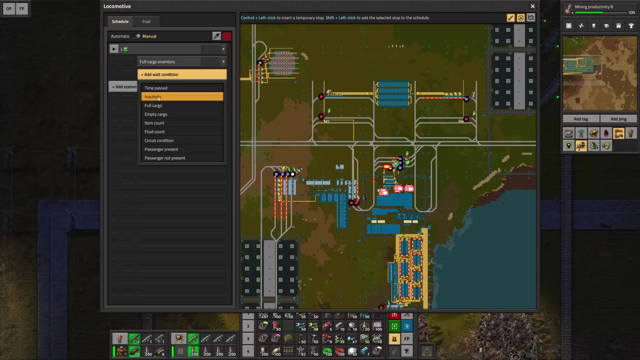 because this one here is gonna remain in the station. I know I did not think about that. yeah, I should have given it its own station. well, maybe I'm gonna change that. for now, I'm just gonna make it go endlessly by. uh, let's see loading up the fuel cells until full cargo or inactivity. 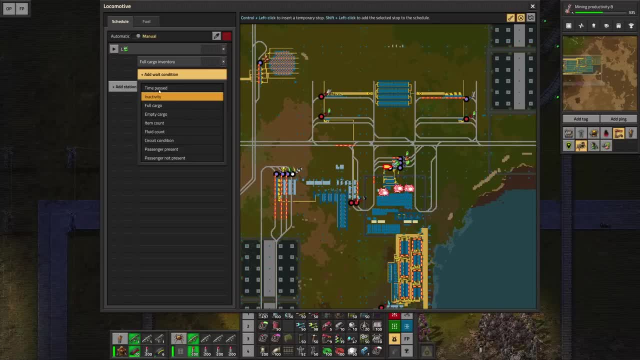 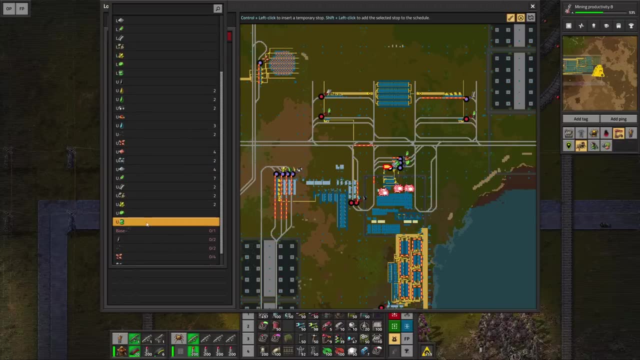 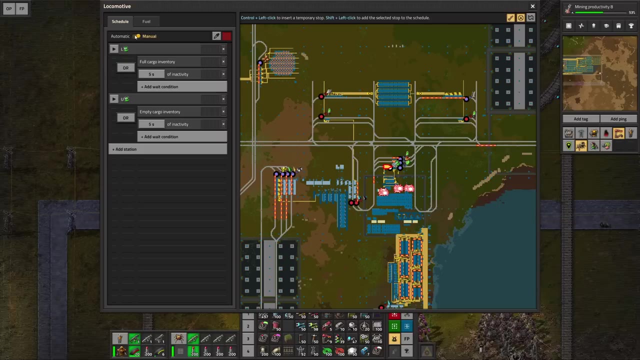 this is how I'm gonna make it still go. it's gonna be a waste of fuel because it's just gonna go back and forth for nothing, but I guess it's fine for now, until I rebuild it. then we wanna unload the fuel cells until empty cargo or inactivity. okay, so let's set this to automatic, and it already goes. 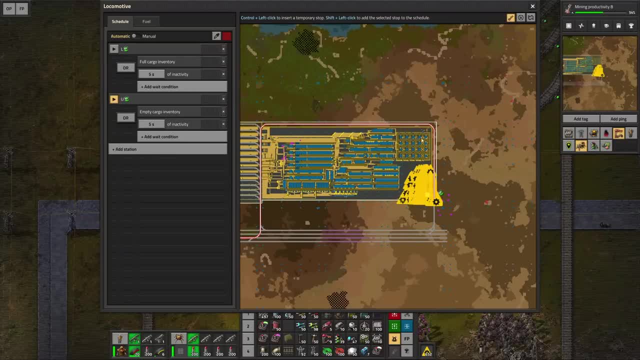 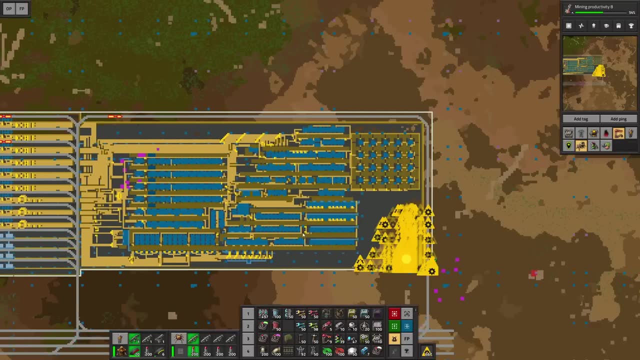 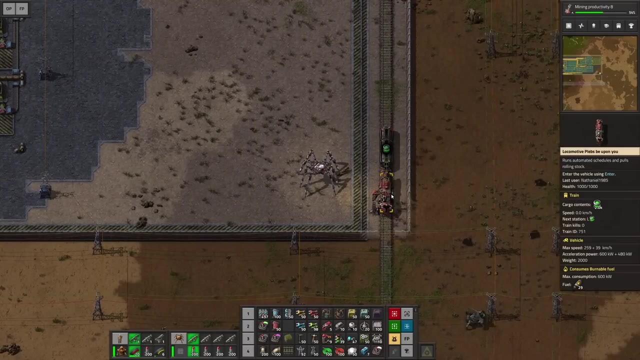 that means it's coming to us right, uh-huh taking the path. okay, this is actually looking fairly decent. it's coming along here, going up and and over nice, and it is already pretty fast. there we go. now we need to unload it. there's gonna be. 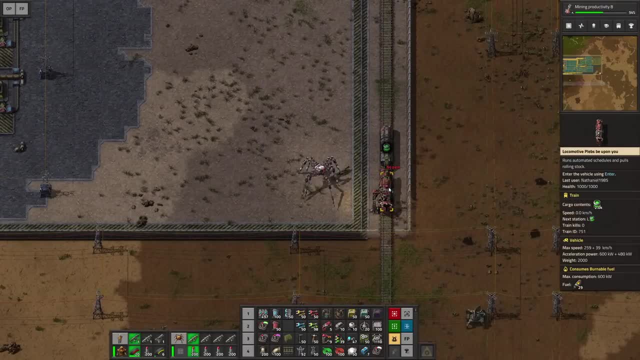 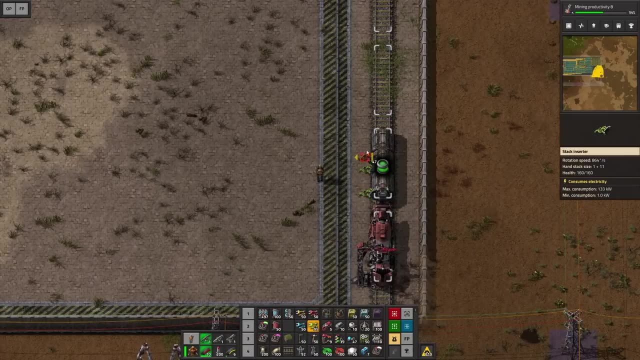 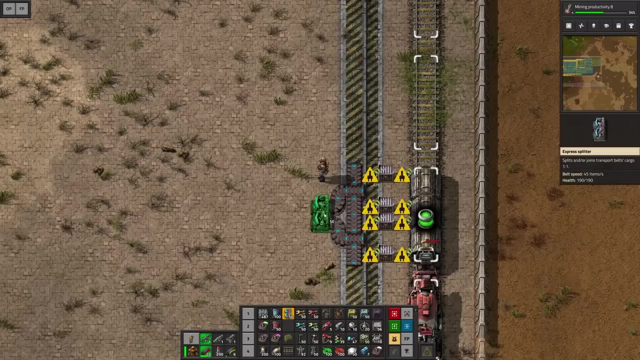 the inactivity right, so it should go again. no path. oh, of course I did not build the rails, but that is fine, it can remain here, because this is where we want to extract it. of course. get those into some storage chests and then over into a belt system, merge these together and now we can use them. 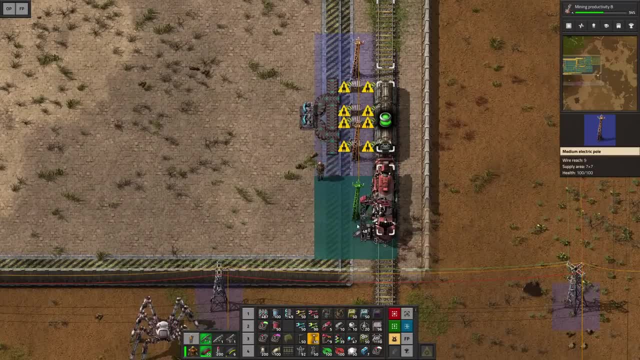 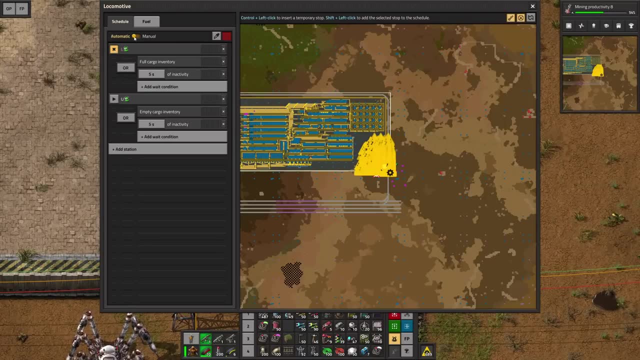 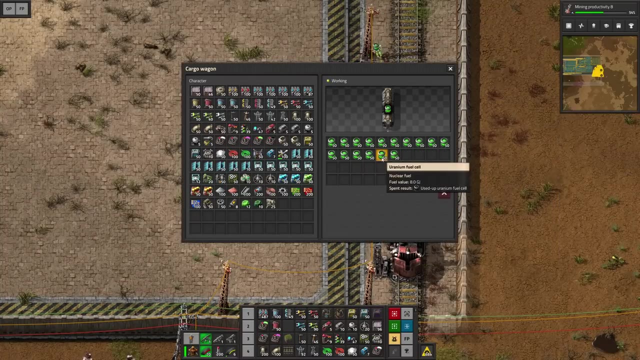 for the nuclear reactor. okay, get this a little bit of power. can we connect it? come on, it won't get unloaded because it's already on its merry way again. uh, can I set it to manual? okay, yeah, that actually worked. now we can first go ahead and empty this and then we can already work with our first fuel there. now go, well, you can't.